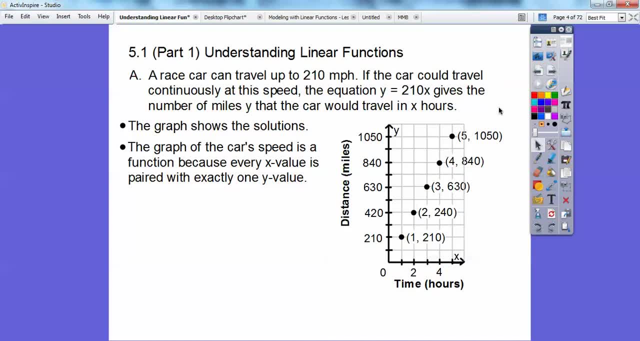 Okay, so it only has one y. right there, There's no points on top of each other, Otherwise it wouldn't be a function right there. Okay, and because the graph is non-vertical, there's no points on top of each other. 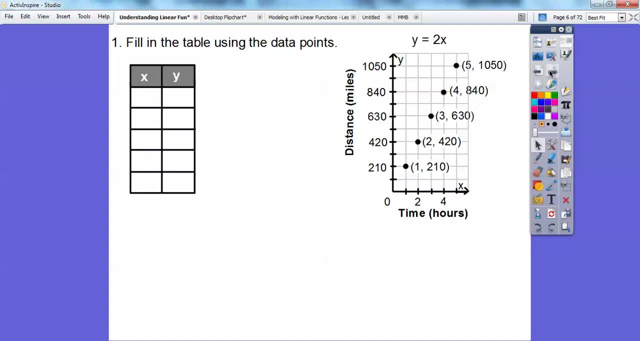 Lines are considered linear functions. Okay, all right, so let's fill in the table using the data points. Okay, so all the x's are all these first numbers: One, two, three, four, five. Okay, all the y's are all these second numbers. 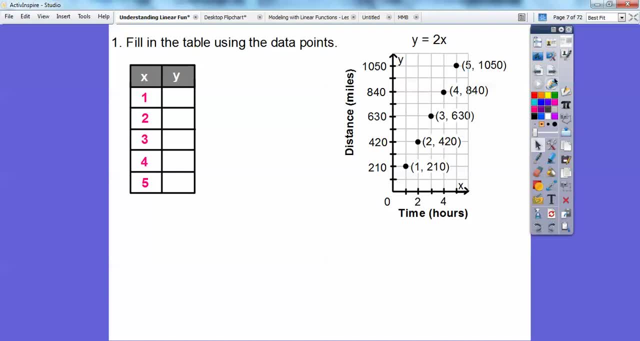 210, 420, 630, 840, 1,050.. Okay, all right, and then, using the table, check that x has a constant change between consecutive terms. So we just want to check that 5 minus 4 is the same as 4 minus 3,. 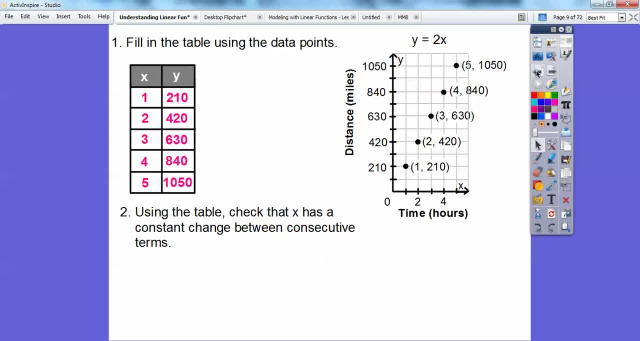 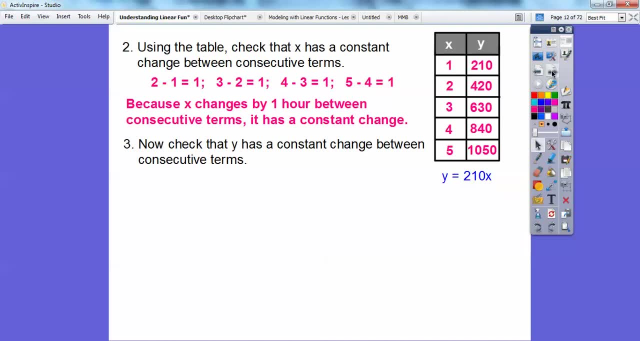 is the same as 3 minus 2, minus 1, and those all equal 1, so they do have a constant change. okay, And same with the y's. Let me just slide that up right here Now. check that the y's has a constant change between consecutive terms. 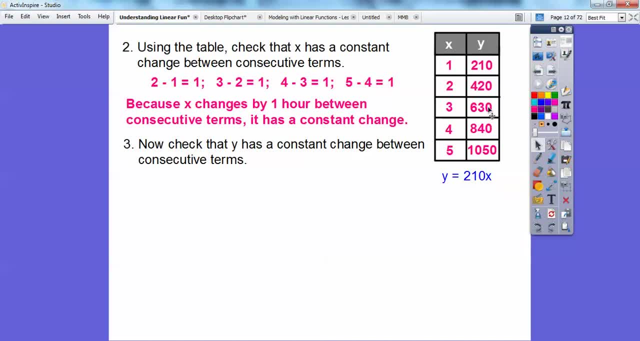 So this term minus this term, this term minus this term, this term minus this term, and so on. So they all equal 210, and so y changes by 210 miles between consecutive terms. so they have a constant change. So using the answers from before, 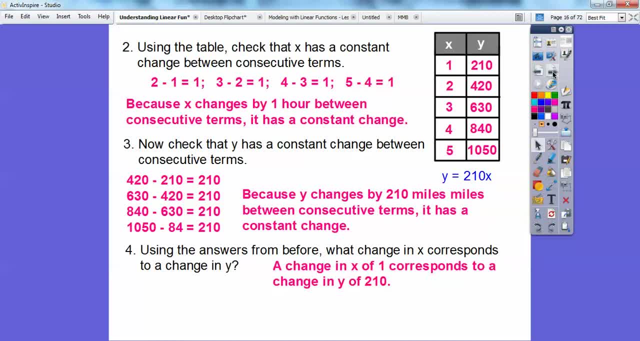 what constant change in x corresponds to a constant change in y. Well, a constant change in x gives us y a constant change of 210.. So, as this goes up by 1,, up by 1,, up by 1, it's making this go up by 210, up by 210, up by 210.. 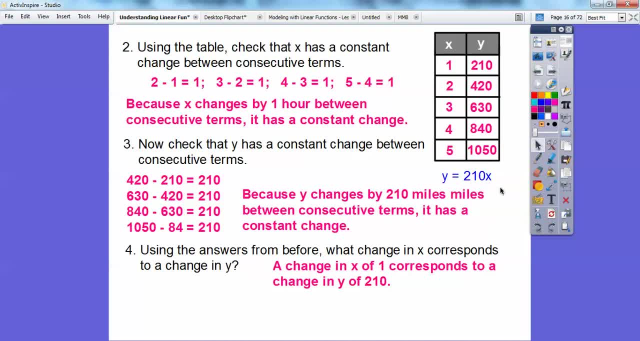 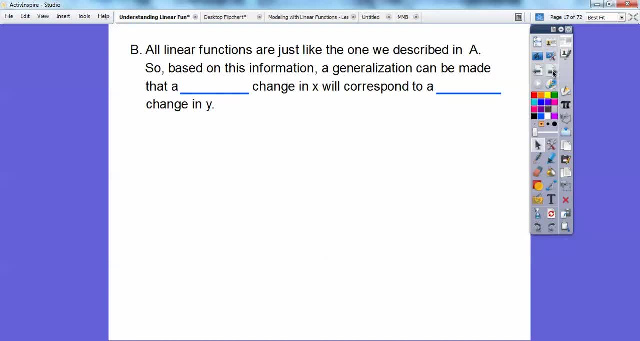 Here's the equation: y equals 210x. okay, So whatever this x value is over here, we multiply it by 210, right there? okay, So all linear functions are just like the one that we just described. So, based on this information, 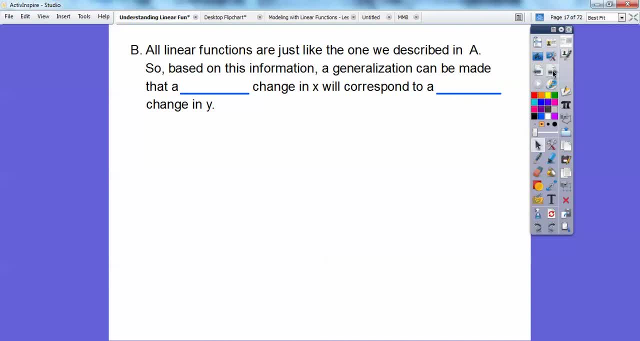 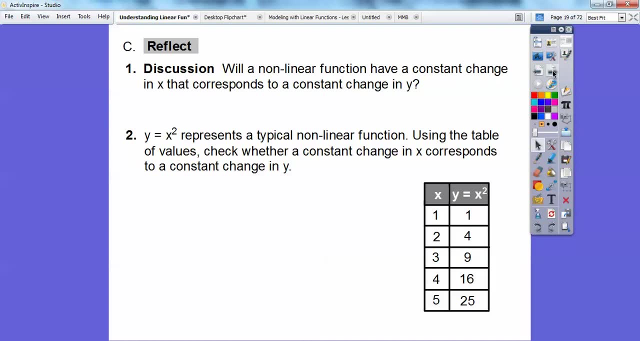 a generalization can be made that a constant change in x corresponds to a constant change in y. That's what happens with linear functions. All right, so will a non-linear function have a constant change in x. that always gives us a constant change in y. 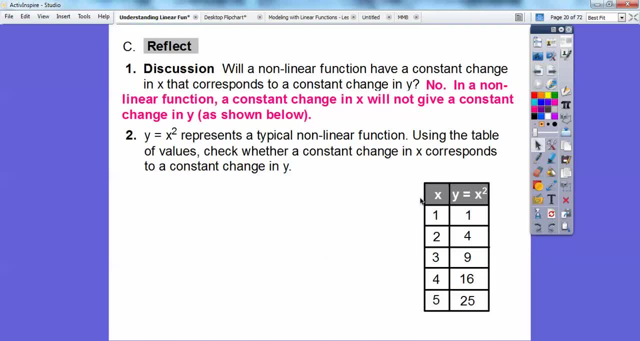 Well, no, it's not going to. We'll show this. one will show us why. Because a constant change in x doesn't give us a constant change in y. So this function is not linear. Okay, so it's called a quadratic. 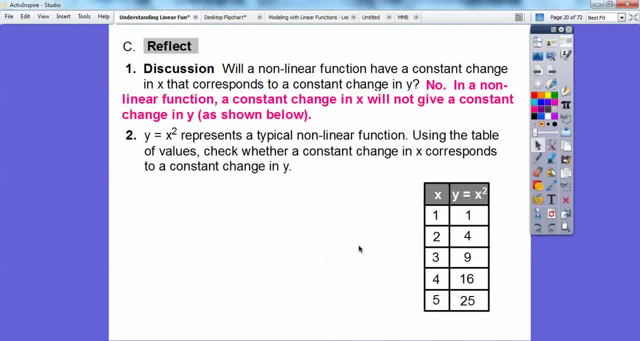 We'll learn how to graph these later, you guys, but it's a parabola when we graph it. But y equals x squared Here, if we plug in x, then 1 squared is 1.. When we plug in x equals 2, 2 squared is 4.. 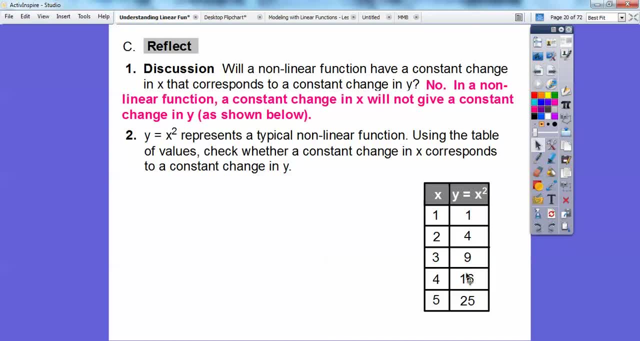 Whoops, I'm going to not answer that phone. 3 squared is 9,, 4 squared is 16,, 5 squared is 25.. That's way across the room. I'm in my classroom right now. It's after school. 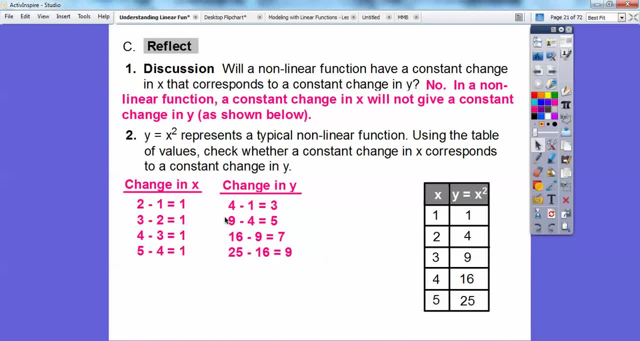 Okay, so look over here, you guys. This constant change in x is 1, and this constant change in y is here. it goes from 3, 4 minus 1 is 3,, so 4 minus 1 is 3,, 9 minus 4 is 5,, 16 minus 9 is 7.. 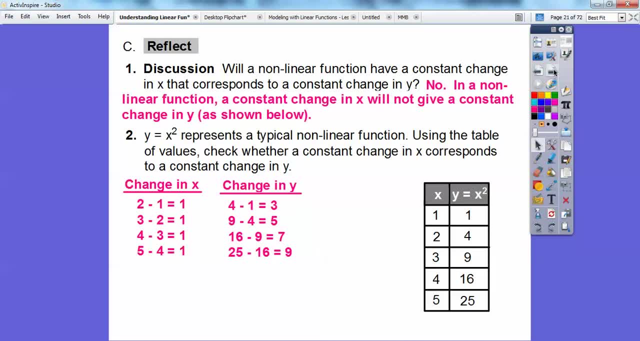 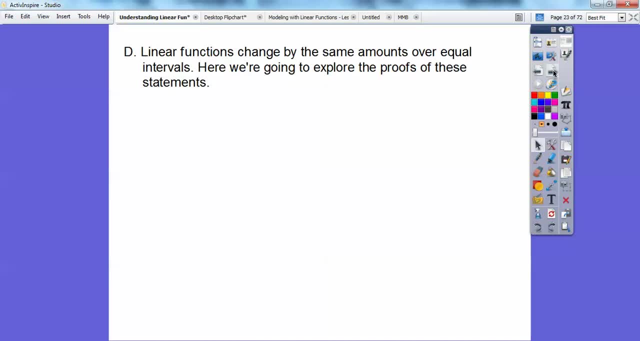 These numbers aren't the same, so they're not constant with each other. So a constant change in x does not give us a constant change in y. Okay, linear functions change by the same amount over equal intervals. So here we're going to explore proofs of these statements. 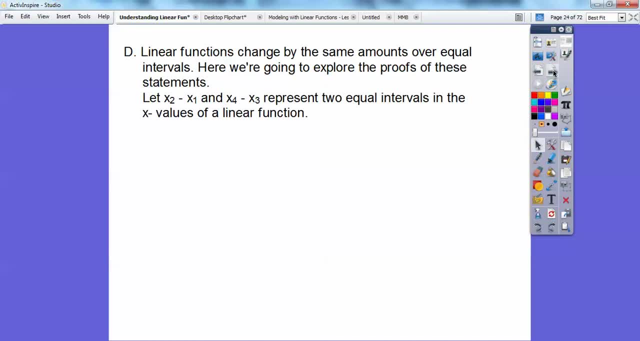 Okay now, if you don't understand this proof, that's okay. Just kind of bear with me for the next minute or so. If I show you a proof, that's in the book right here. okay, you're going to be doing proofs later on. 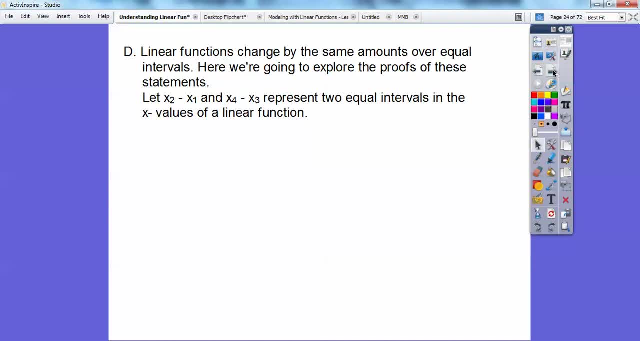 I think it's more integrated too, but here's our first proof. okay, So let's just pretend like the second x minus the first x and the second or the fourth x minus the third x represent two equal intervals in the x values, okay? 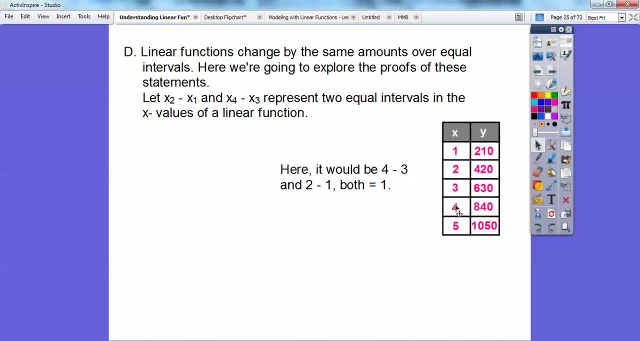 So here it would be. here's the fourth x minus the third x, and here's the second x minus the the first x, and they both equal one when we subtract those right here. okay, We need to recognize also that f of x equals mx plus b. 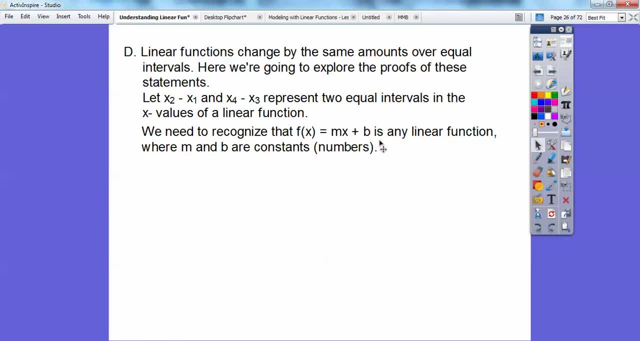 Remember this is like y, right here, y equals mx plus b. is any linear function? okay, We'll talk about this in a little bit. That's called slope intercept, where m and b are just constant numbers. m is our slope, we'll learn later. 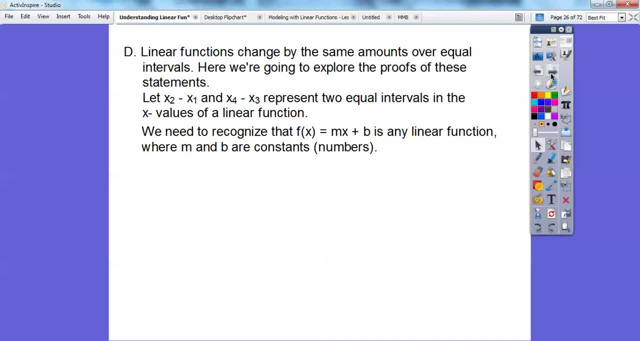 and b is our y intercept. we'll learn later, but they're just numbers. okay, So we're going to complete the proof that linear functions grow by equal differences over equal intervals. okay, So we're going to start with that. these guys are equal. 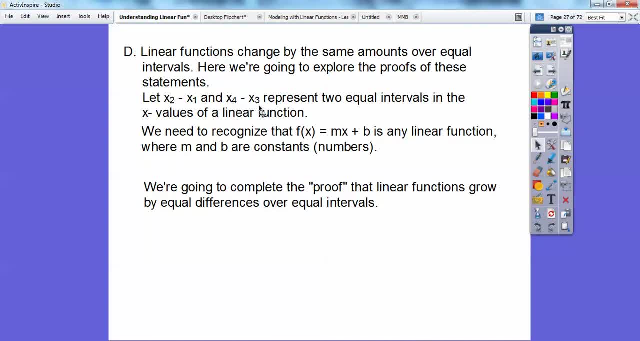 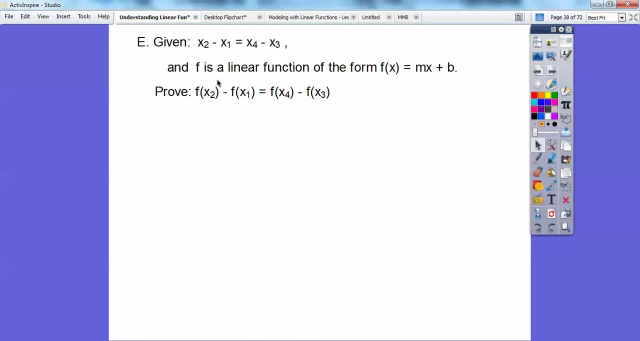 The second, x minus the first, is going to equal the fourth minus the third right here. Okay, so here's how proofs look. They give us this given information. okay, And this is given also. f is a linear function of the form. f of x equals mx plus b. 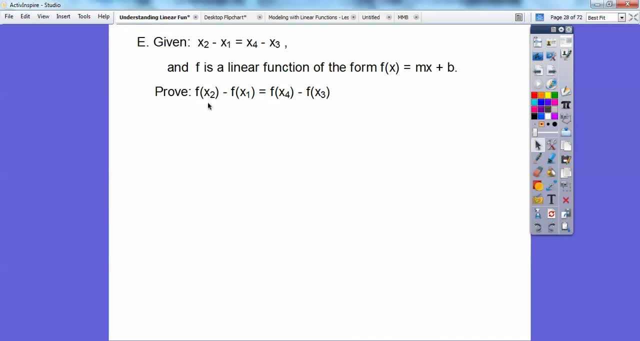 Remember, y equals mx plus b. We're just going to prove that. remember this: f of x is y. so this is like saying our second y minus our first y is going to equal our fourth y minus our third y. So, given that x, the second x minus the first x, 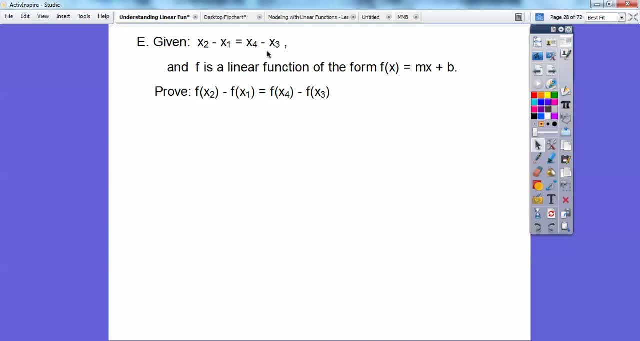 equals the fourth x minus the third x. we're going to prove that the second y minus the first y is going to equal the fourth y minus the third y. Now, if you don't understand this, that's okay, You can hang in there. 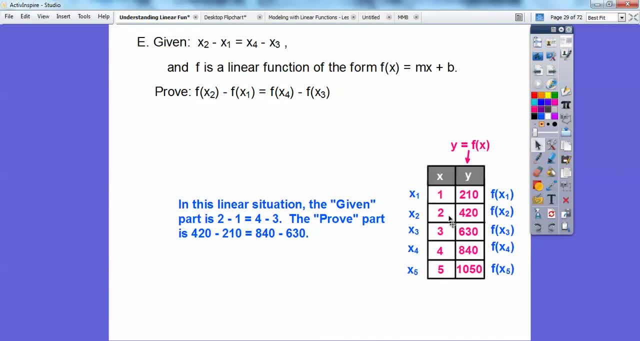 Okay, so in this linear situation, here's the second x minus the first x and here's the second y minus the first y. right here, Here is the fourth y minus the fourth x minus the third x. Here's the fourth y minus the third y. okay. 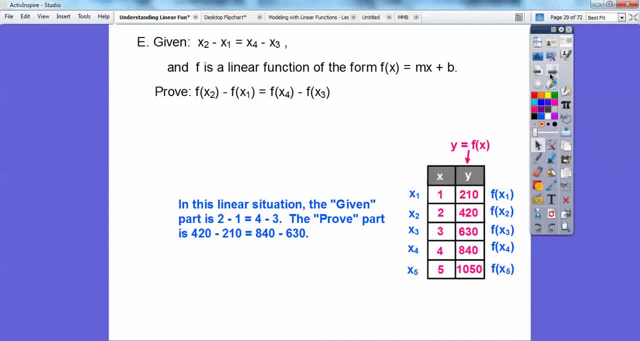 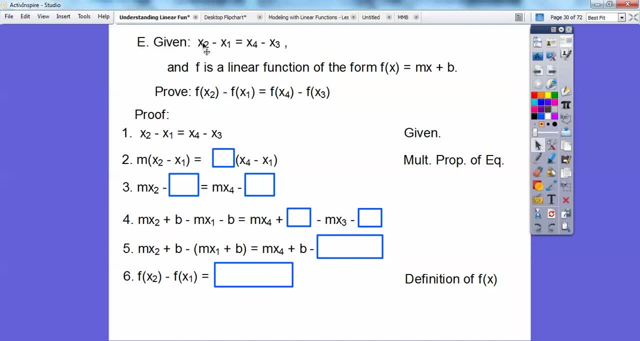 That's all this mumbo jumbo. right here is stating: right there, okay, All right, and then you see that ugly thing right there, okay, Now look right here. here's the given information. that always starts at the top, okay. 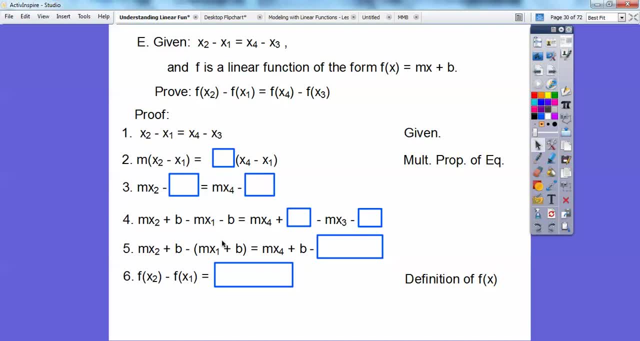 And the prove statement is always going at the bottom of prove. So here's this half right here, okay, And this half is going to go right here, okay, All right, Let's just do this one at a time, because it's overwhelming when you see it like that. okay, 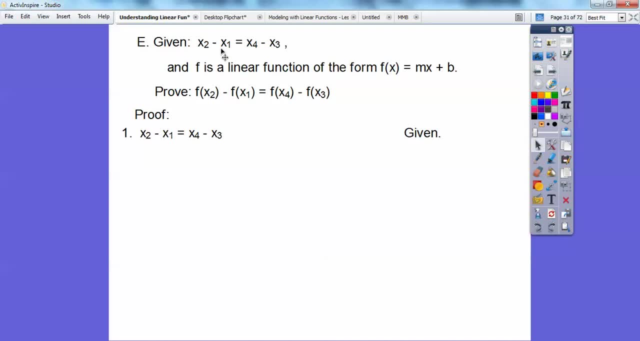 So are you guys? okay, right there, This is given right here. They gave us that information right there, All right. so what happened to this right here? Well, here, we just plugged in m on both sides. We just multiplied both sides by m. 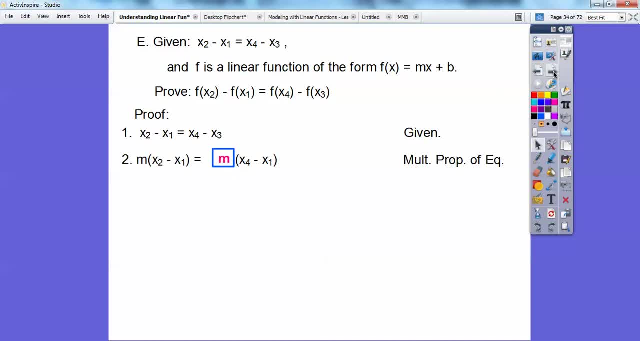 So I'm going to put an m right there and call it the multiplication property, right there? okay, Now check this out right here. Here. what they did is they put this m through: m times x sub 2 minus m times x sub 1 will go right here. 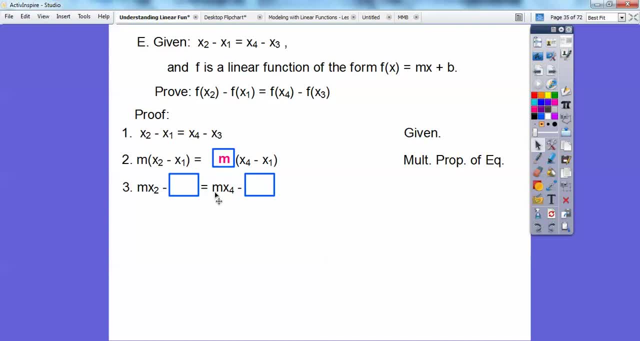 It's going to equal m times x sub 4, that's what this says right here- minus m times x sub 1.. That's what's going to go in right there, okay, And what is that called? That's called the distributive property. 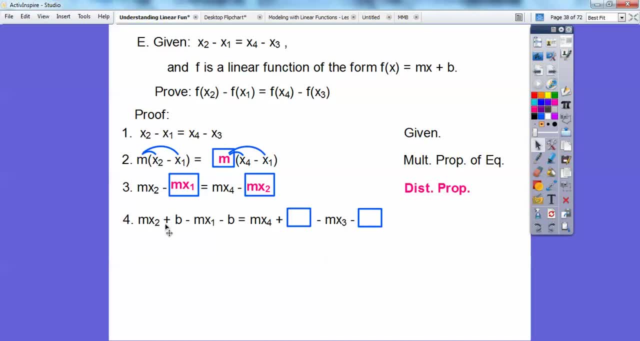 All right, okay now look. All they did right here is they just added a b and they subtracted a b. right there, okay? So we're going to do the same and add a b and subtract a b. All we did is we added b and subtracted b from both sides. 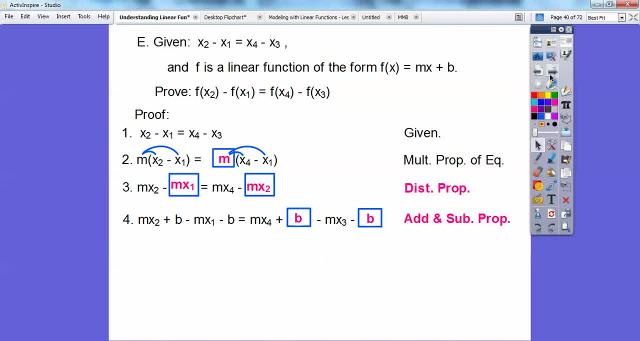 So the addition and subtraction property: added and subtracted the b's. okay, All right, and then. so here, what they did was is they pulled the negative out of this and this. So here it is. Imagine if I redistributed this negative through. 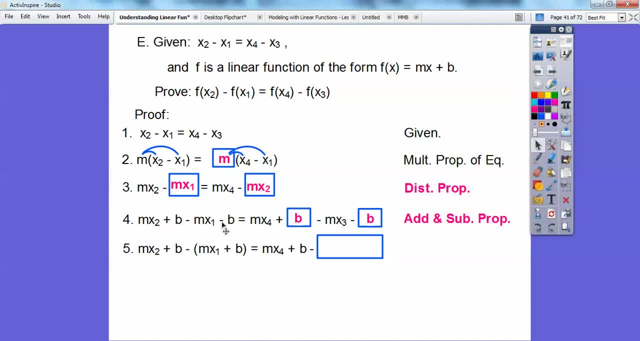 it would get me to there and put this negative right there. it would get me there. Okay, so that's all they did. right here is they pulled the negative out of here, So this is going to be positive. m x sub 3. 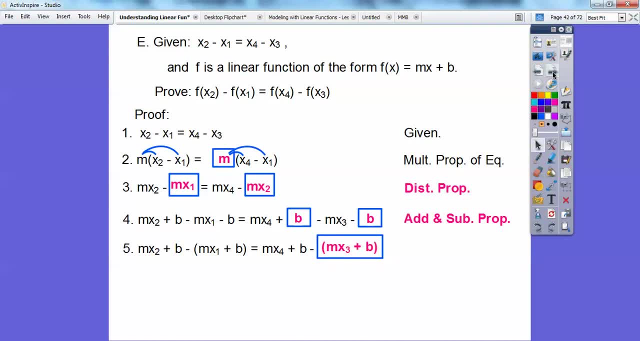 and this is going to be plus b, right there, okay, And that's called the distributive property. It's like the reverse distributive property. All right, you guys? okay, so here's mx plus b. This is part of the given right here. 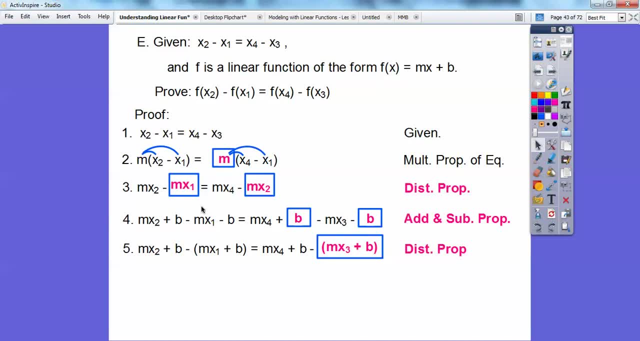 This equals f of x. okay, So here's mx sub 2 plus b. So this is going to be equal to f of x sub 2.. Look there, it is right there. This is mx sub 1 plus b. So here's mx plus b. 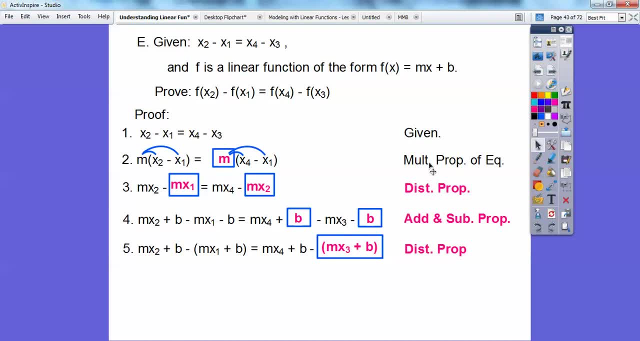 So this must be f of x sub 1, okay, So that's what that is, right there, okay, And then check this out. Here's mx sub 4 plus b. okay, That's just f of x. so this is going to be f of x sub 4.. 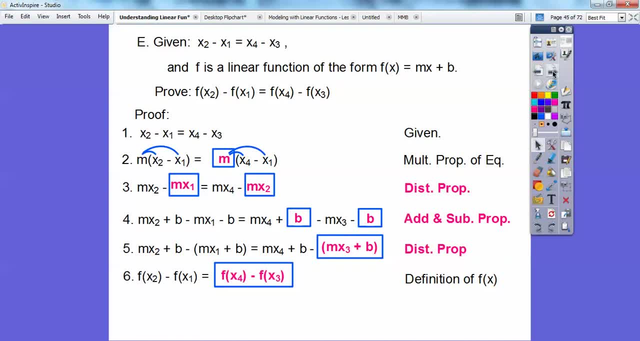 And this is going to be minus f of x, sub 3,. okay, Now, if you didn't get that, don't worry about it, you guys. Let's get back to the math here. So consider the function: y equals x, cubed. 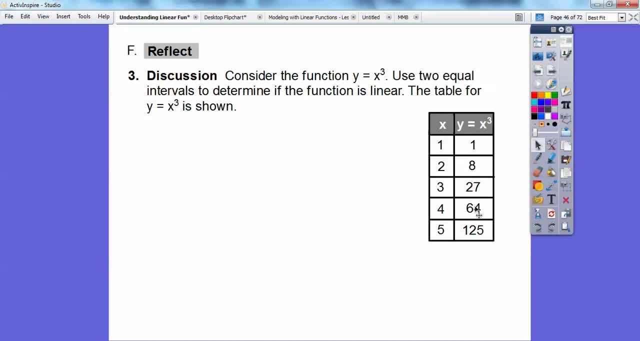 Here's 1 cubed, here's 2 cubed, here's 3 times 3 times 3, 4 times 4 times 4, here's 5 cubed, right here, okay, So here's y equals x cubed. 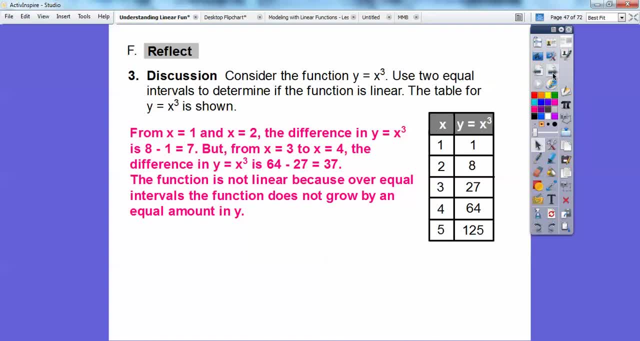 So the table? so is this function linear? So from x equal 1 to x equal 2, right here it goes up by 1.. But check this out, This jumps up by 2.. This goes up by 7,. okay. 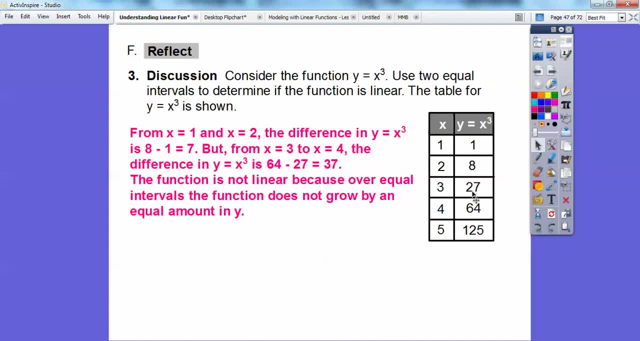 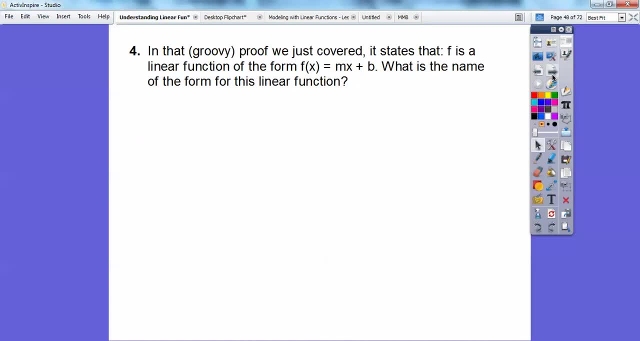 And then we go from 3 to 4. It goes up by 1, but this goes up by 37 over here. So it's not a constant change. so this function is not linear because it's not a constant change, all right, 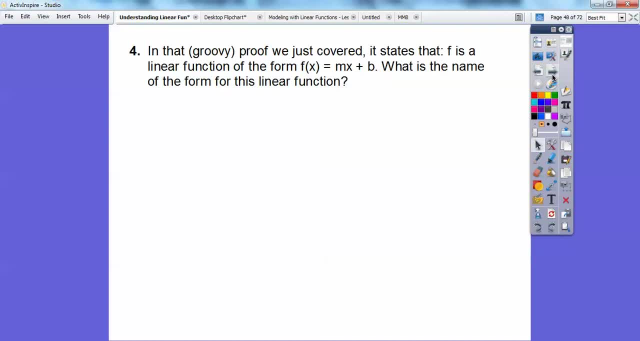 So in that groovy proof that we just covered, it states that f is a linear function of the form f of x equals mx plus b. Do you remember what this is called right here? That's called slope intercept form of a linear equation. 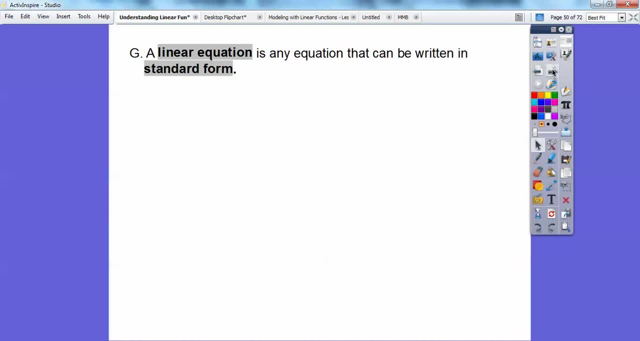 All right. a linear equation is any equation that can be written also in standard form. Standard form is ax plus by equals c, And this a, this b, this c are real numbers, and both a and b can't be 0.. 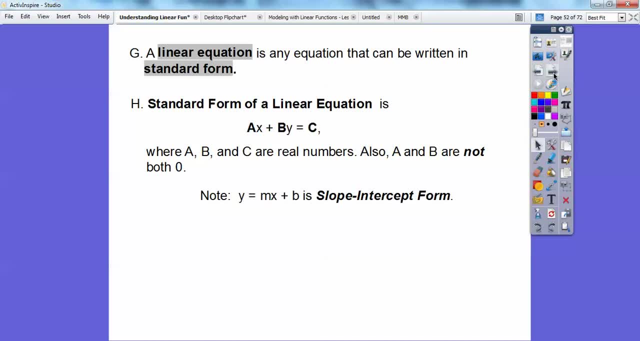 a could be 0 or b could be 0,, but they both can't be 0,. okay, And y equals mx plus b is slope intercept form. All right, so determine whether the equation is linear. So graph the function. We'll be done with this in just a second. 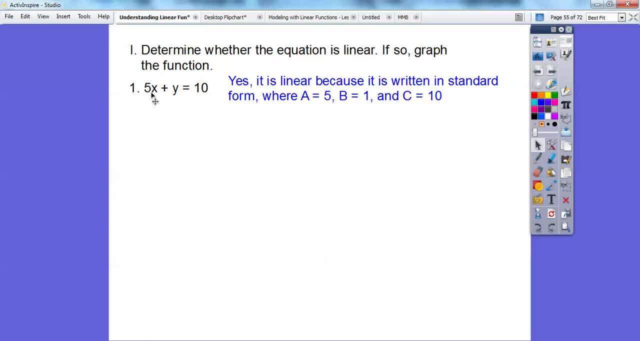 So is this linear? Yeah, that's in standard form, right there, and we're going to add 5x, plus there's a hidden 1 right there by equals c. So a is 5, b is 1, and c. is that 10, right there? 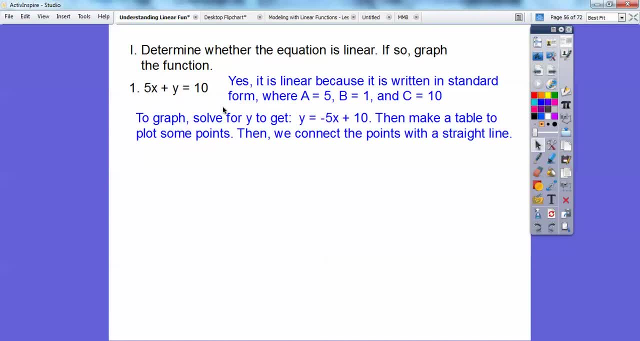 All right. so if we solve for y, we just subtract 5x from both sides and then we'll make a table and plug in the points right here. okay, So we're going to plug in negative 1 right here. Negative 5 times negative 1 is positive 5.. 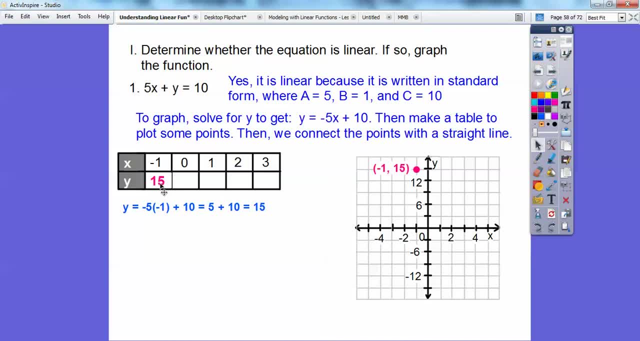 And when we add 5 plus that 10, right there it gets us 15.. So here's negative 1 comma, 15, right here. Okay, let's plug in 0. Negative 5 times 0 is 0, plus 10 is 10.. 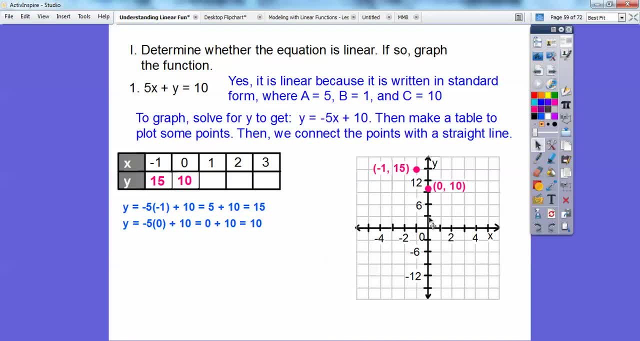 Here's 0, 10 right there. okay, It looks like these tick marks are going by 3s. There's 3,, 6,, 9,, 12.. Okay, let's plug in 1.. Negative 5 times 1 plus 10 is 5, okay. 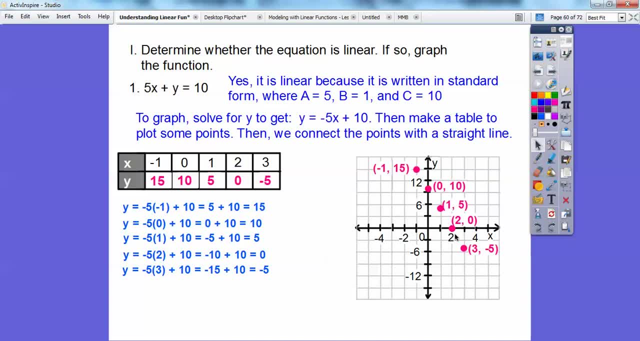 And there's the rest of them. Look, it makes a nice straight line right there. okay, So it is a linear equation. So always we write the equation next to the line. So we're going to be doing several lines, And so we always write the equation somewhere by the graph. 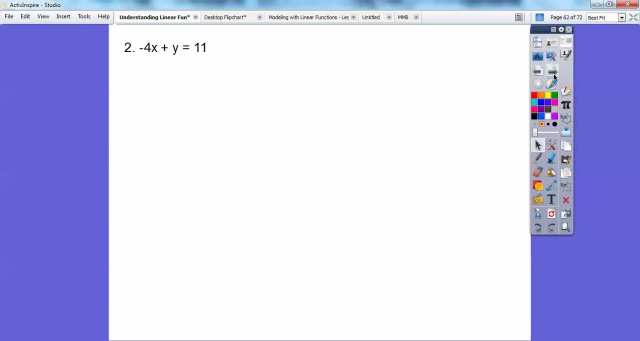 of where we're doing that, Let's try another one. Okay, is this in standard form? Yes, it is. It's in standard form, And a is negative 4,, b is that 1, and c is 11..